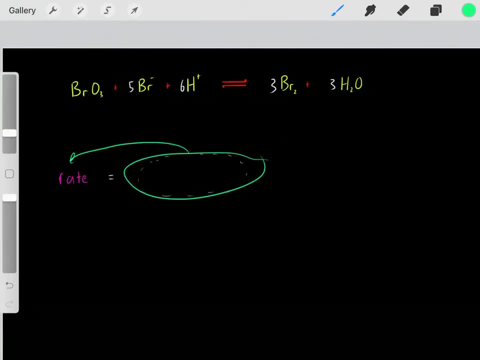 of this chemical reaction. What are the terms that affect the rate of this chemical reaction? Well, we know the rate constant is important. We explained: the higher the rate constant, the larger the rate constant, the faster the rate. So the rate constant of this chemical. 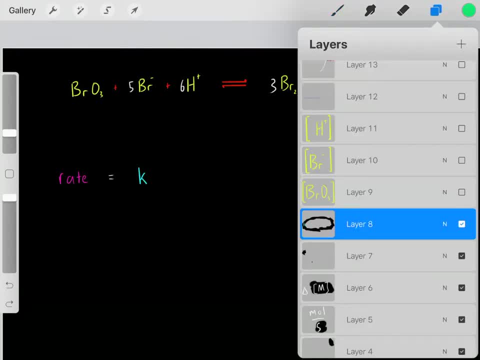 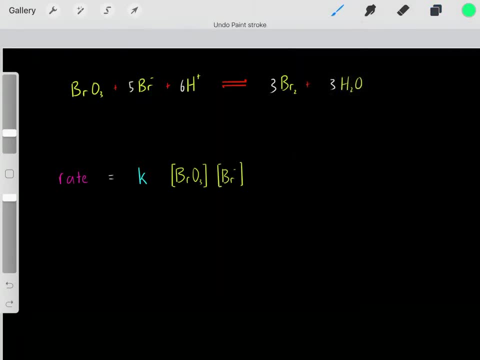 reaction has an impact on the rate. But what else? Well, we also know the concentration of this reactant will have an impact on the rate, And also this reactant—this is another reactant whose concentration will impact the rate, also this reactant. These are all reactants whose concentrations will impact the rate of this. 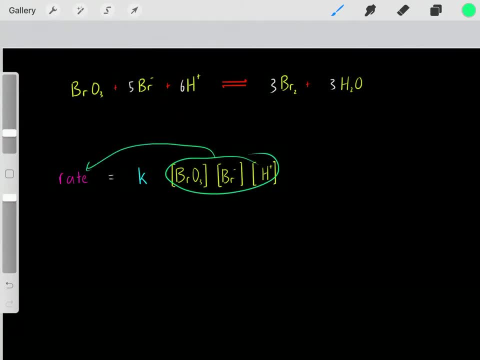 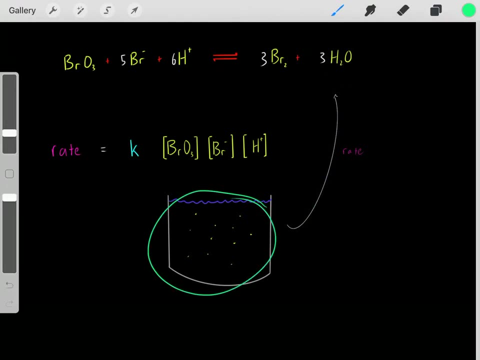 chemical reaction. So therefore they will impact the rate of the reaction. So they should be involved in this equation. And this makes sense because, if you think about it, let's say we had the solution with all these reactants, Let's say we had all these reactants in the solution And 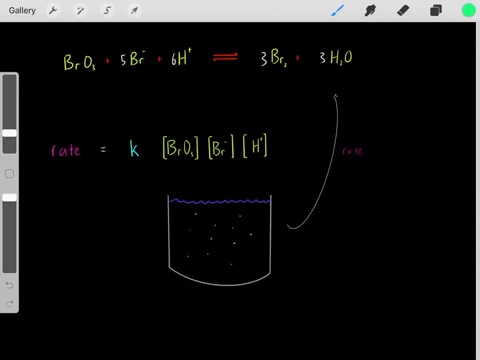 let's say we had a small concentration of all the reactants. Yeah, we know they're going to react. They're going to randomly bump into each other And when they bump into each other they're going to react, forming products. So we have a small concentration of all reactants. They're going to 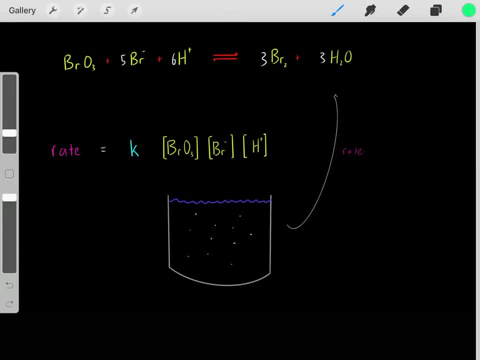 react, and we're going to have a certain rate. They're going to react and we're going to have a certain rate of products being formed. However, what happens if we increase the concentration? Now, let's say we dramatically increase the concentration. What's going to happen? 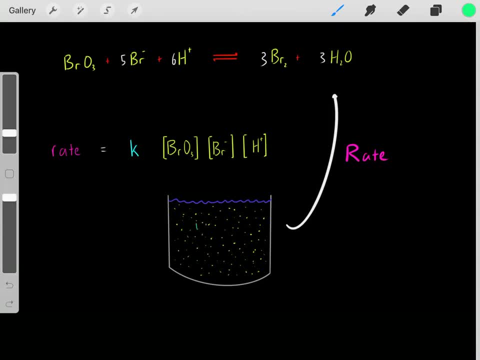 Well, now we're going to have more interactions, We're going to have more random collisions, So we're going to have more reactions occurring per second. So we're going to have an increased rate. We're going to have more molds of products made per second. 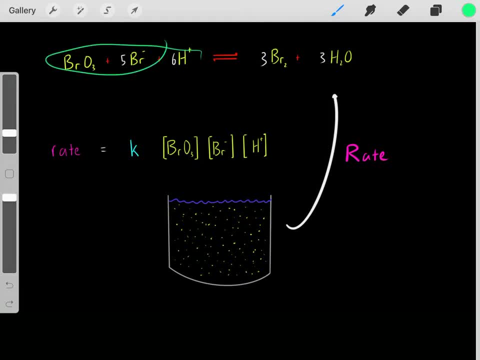 So we're going to have a faster rate. So therefore we see the concentration of these reactants impact the rate of the reaction. If we have a high concentration of our reactants, we'll have a high rate of the reaction. So it's the concentration of the reactants that impact. 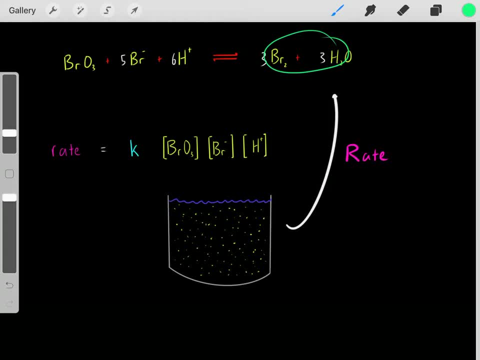 the rate. We know the concentration of the products have no impact on the rate of the chemical reaction. Why would they impact? So therefore they're not involved in this equation. It's only the concentration of the reactants that impact the rate of the reaction. So it's. 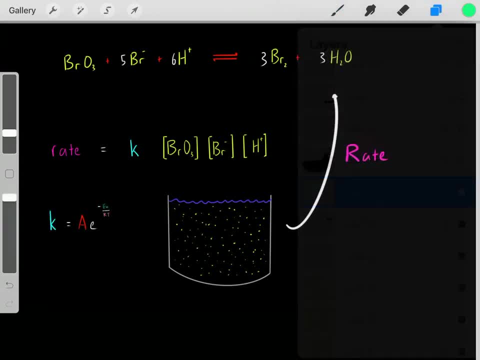 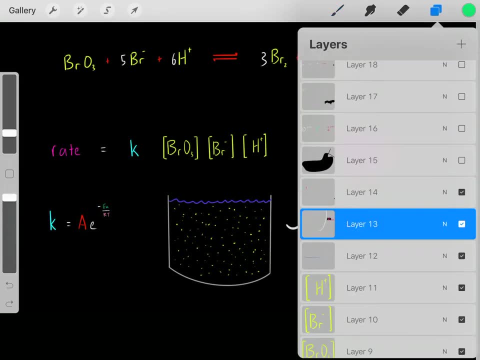 the concentration of the reactants that impact the rate of the reaction And again, the rate constant. We explained the rate constant impacts the rate of the reaction And we can determine the rate constant using this equation. So now that we know this, let's go into more details on exactly what's happening. So this 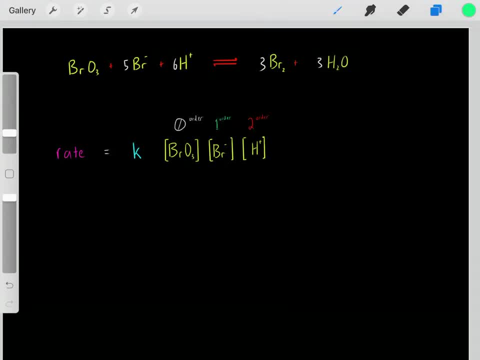 describes the rate of this reaction. But something important to realize is a reactant can either be zero order in the way it affects the rate of the reaction, It can be first order in the way it affects the rate of the reaction, Or it can be second order in the way it affects the rate of. 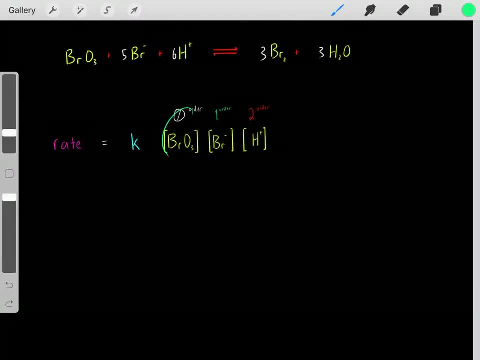 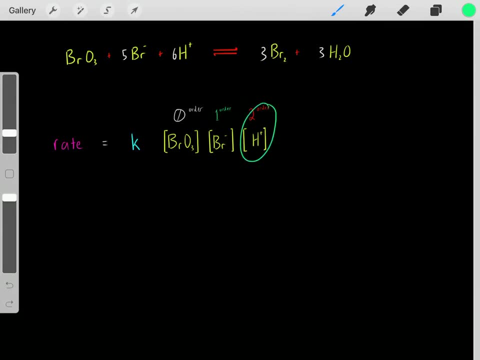 the reaction. So in this video, just for simplicity, let's say that this reactant is zero order in the way it affects the rate of the reaction, Let's say this reactant is first order And let's say this reactant is second order in the way it affects the rate of the reaction. So I'm just going to do one. 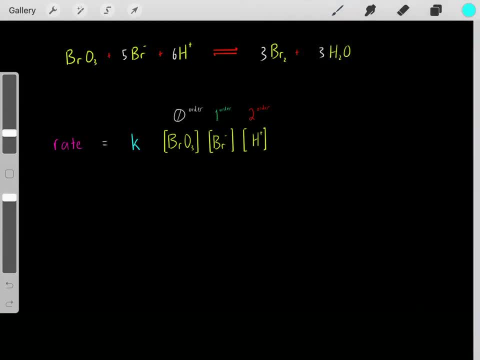 of each example just to illustrate exactly what's going on. So what does it mean if this reactant is zero order in the way it affects the rate of the reaction? Well, really, what it means is that it actually, the concentration of this reactant- doesn't affect the rate of the reaction. That's. 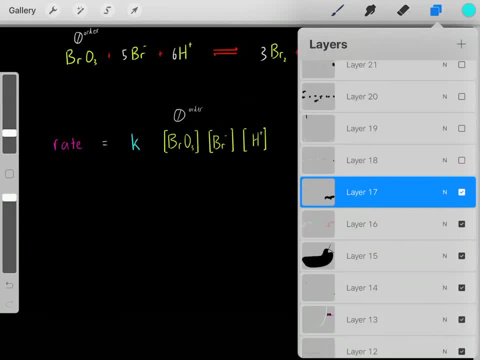 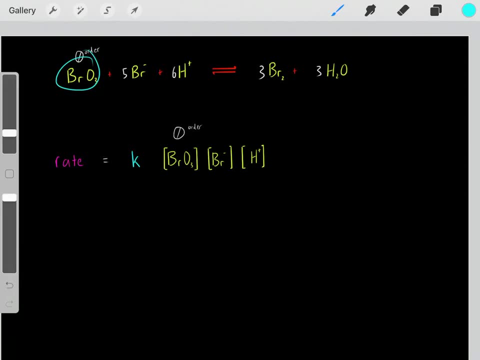 what it means. So, for example, let's say, we know this reactant is zero order in the way it affects the rate of the reaction. So therefore the concentration of this reactant doesn't affect the rate of the reaction. For example, let's say we did an experiment where we had one molar of this guy, one molar of this. 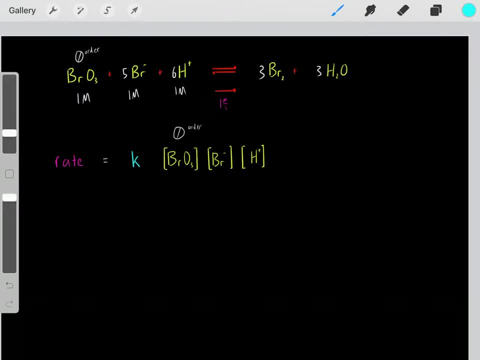 guy and one molar of this guy. So let's say, under these conditions, we had this rate: one molar per second of products being made per second with this particular rate. However, now let's do another experiment where we double the concentration. So now, instead of one molar, let's say we have 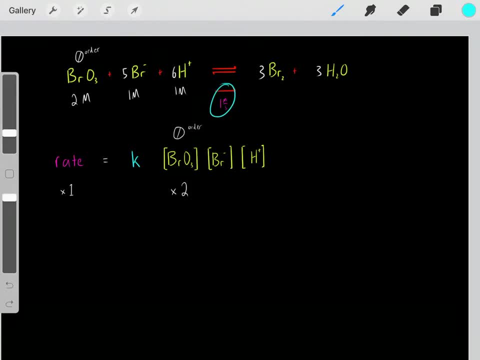 two molar of this guy, we would have the same rate of the reaction. We would still have one molar per second. So therefore, we saw, when we had this, these concentrations, we had this rate. But when we double this concentration, we still. we double the concentration, we still have the. 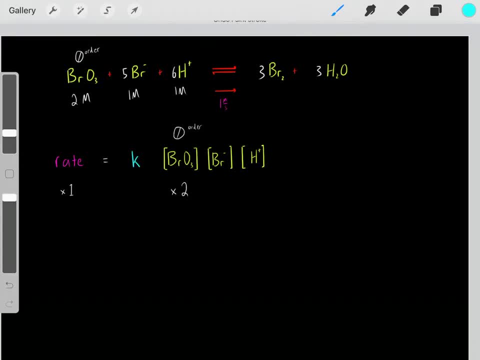 exact same rate. So therefore we know this reactant is zero order in the way it affects the rate of the reaction. It doesn't affect the rate of the reaction. And a way you can describe that is: if you double the concentration of this reactant, you multiply the rate of the. 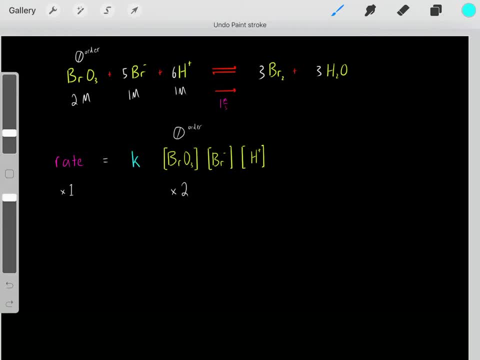 reaction by one. So, therefore, which means it had no effect on the rate of the reaction. But now let's say this reactant is first order in the way its concentration affects the rate of the reaction. So what does that mean? Well, let's do an experiment. Let's say we had one. 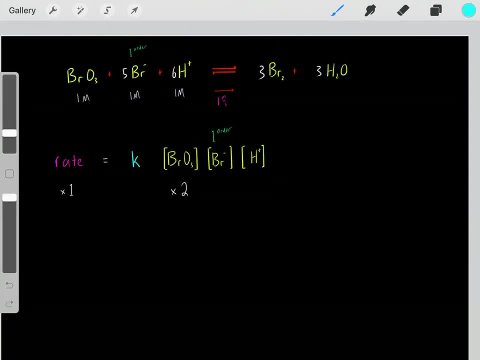 molar of all these reactants and they reacted and we had a rate of one molar per second. Now let's do another experiment where we double the concentration of this reactant. What's going to happen if we double the rate of the concentration of this reactant? Well then, we'll double the rate. 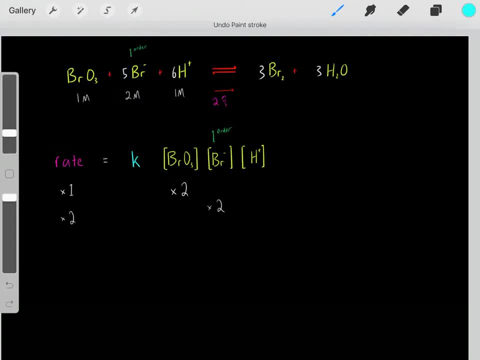 of the reaction. So in this example, this guy's concentration did impact the rate of the reaction. Remember, when we were at one molar of all these guys, we had this rate. However, when we double this concentration, we doubled the rate. Now we have two molar per second rate of the reaction. So under these, 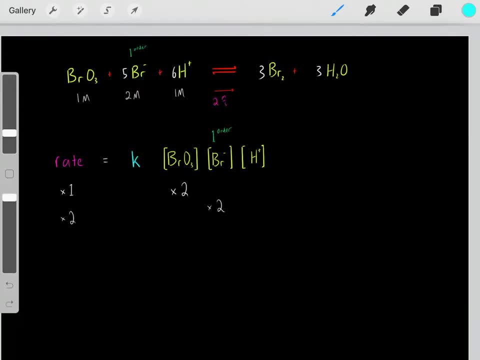 circumstances. therefore, this guy must be first order in the way it affects the rate of the reaction, which means the concentration of this guy does impact the rate of the reaction. As we double the concentration of this reactant, we double the concentration And again, a way you 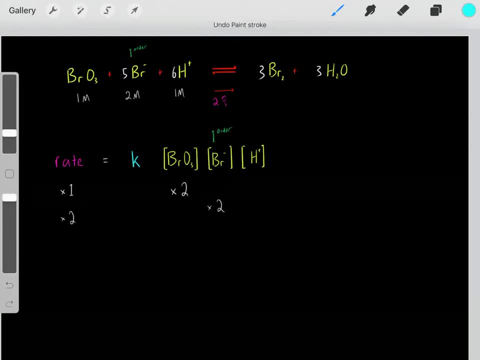 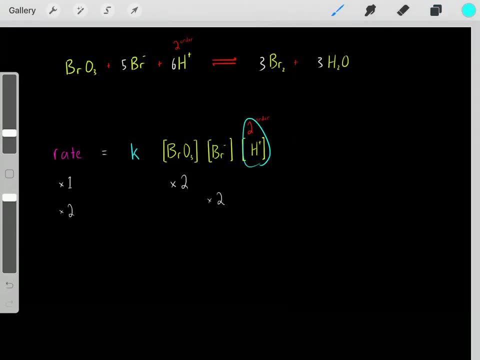 can describe. that is, if you double the rate of the reaction, you double the rate of the reaction is, if you double the concentration of this reactant, you double the rate. So when you see that, that means it's first order. So what about this guy? Let's say, this guy happens to be second. 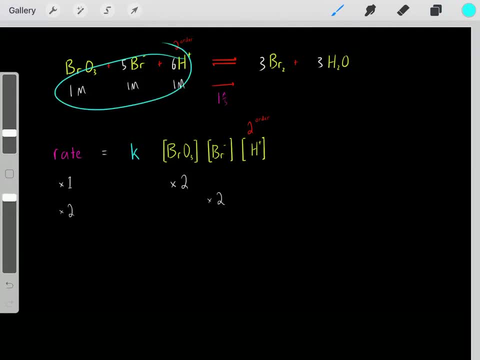 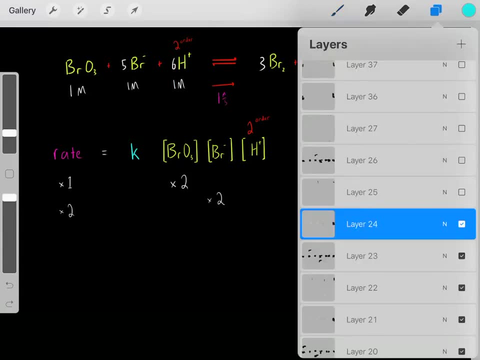 order. What does that mean? Well, we can do an experiment: one molar concentration of all reactants, and let's say we had this rate, this rate one moles per second. But now let's say we double this guy's concentration. What's going to happen? Well, if we double this guy's concentration, 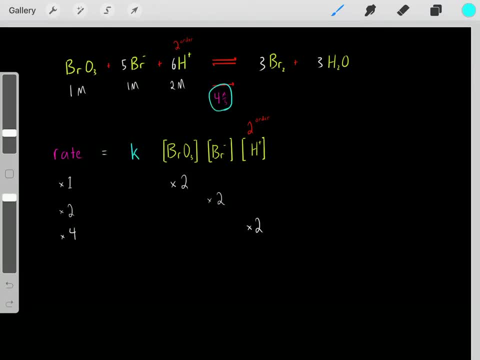 now we quadruple the rate of the reaction. Now the reaction is at four molar per second. So we see this guy's concentration has a big impact on the rate of the reaction. Originally when we were at one molar, we are at one moles per second. But when we doubled this, 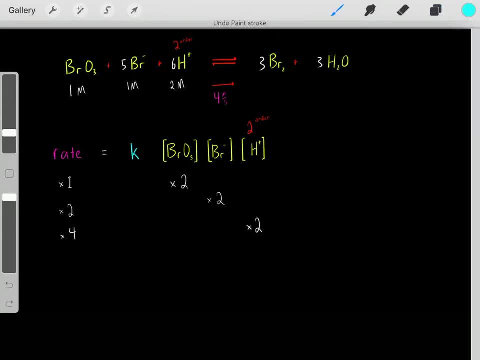 concentration, we quadrupled the rate of the reaction. So therefore this guy's second order, in the way it affects the rate of the reaction, the rate of this reaction is very sensitive to this guy's concentration Because, again, this reactant is second order. So if you double the, 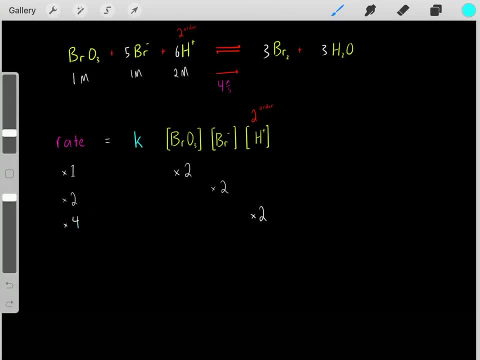 concentration of this reactant, you quadruple the rate of the reaction. So therefore there are different ways to calculate the rate of the reaction And the way to do that is to different ways these reactants' concentration can impact the rate of the reaction. If you're 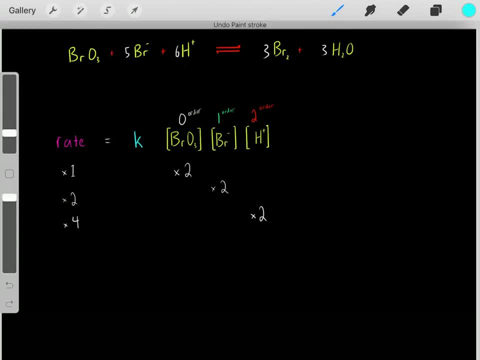 zero order, the concentration of that reactant doesn't impact the rate of the reaction. If it's first order, then if you double the concentration of this reactant, you double the rate of the reaction. If it's second order, if you double the concentration of this reactant, you quadruple the. 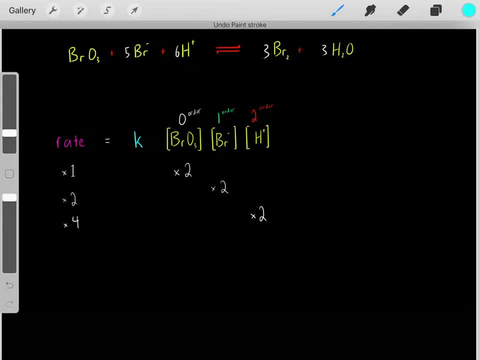 rate of the reaction. And why is this called zero order? first order, second order. Well, you can complete the pattern and see: If you multiply the concentration of this guy by two, you multiply the rate by one, And two to the zeroth power is one. If you double the, 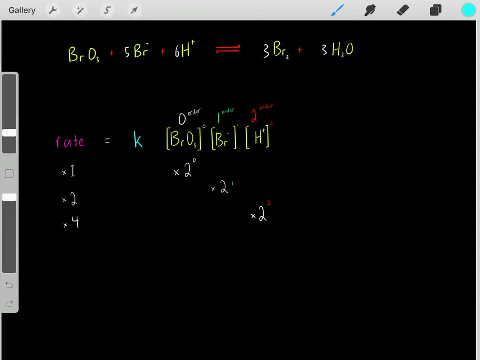 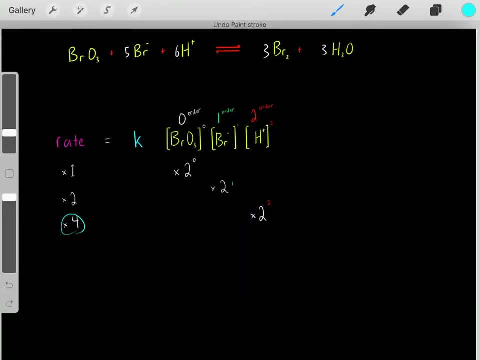 concentration of this guy, you double the rate of the reaction, And again, times two to the first power equals two. And again, if you double the concentration of this guy, you quadruple the rate of this reaction, And again you multiply this. and then, because it's second order to the 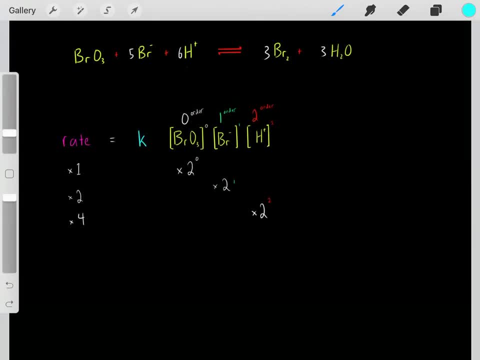 second power, that's four. So that's just the theme And again, so you can just connect this pattern. But the point is there are different ways the concentration of these reactants can impact the rate of the reaction. And if you're zero order, then if you double the concentration, 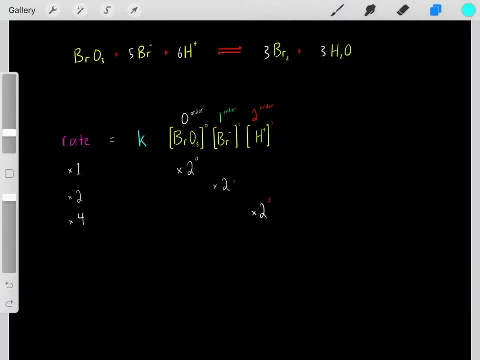 of this guy, you quadruple the rate of the reaction. And again, really to illustrate what's going on, remember this guy's first order. So if you double the concentration, you double the rate of the reaction, But notice the pattern. So, for example, maybe we quadruple the concentration of 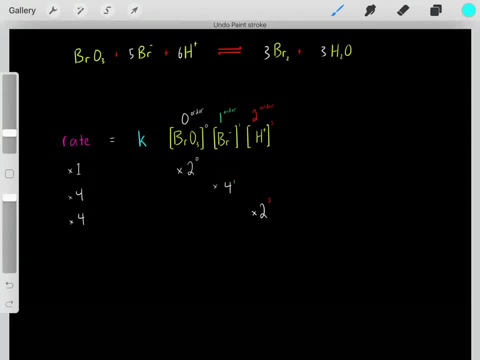 this guy, this reactant, then you would quadruple the rate of the reaction Because, again this pattern, it would go to the first power because it's first order. So therefore, four to the first power is four. And what about this guy? We said it's second order. So therefore, if you double, 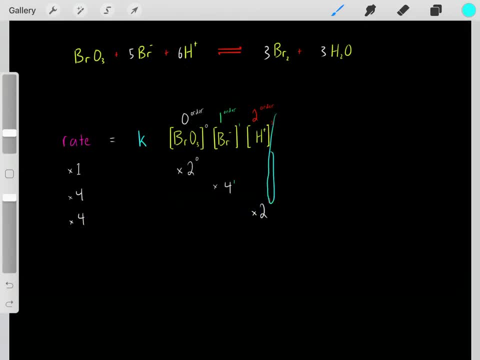 the concentration of this reactant, you quadruple the rate of the reaction because it's second order. So if you double the concentration of this reactant, you quadruple the rate of the reaction Because again that pattern. So maybe we do another example. Maybe we multiply by three the. 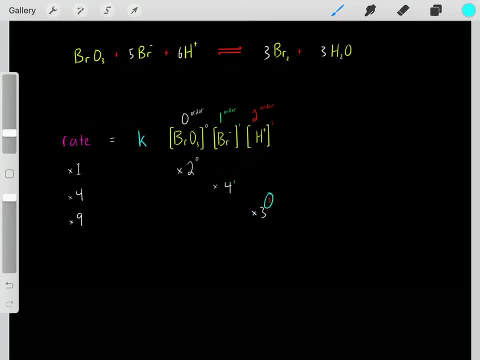 concentration of this reactant. Then again we now do the pattern. We would see we would multiply the rate of the reaction by nine, Because again it's this pattern. If it's second order, then just notice this pattern. But again, the point is there are different ways that these reactants can impact. 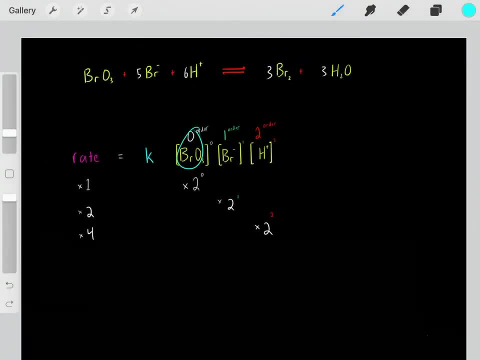 the rate of the reaction. And if you're zero order, the concentration of that reactant has no impact on the rate of the reaction, and et cetera. So these are the two patterns. These are the three common ways the concentration of a particular reactant can impact the rate. 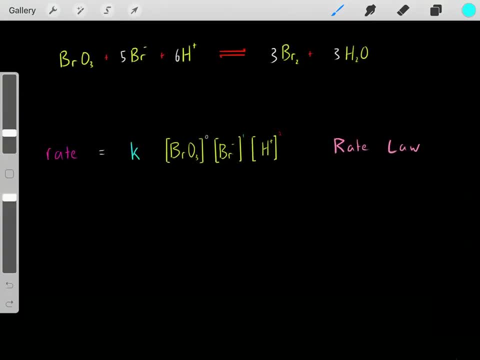 of the reaction. So this is referred to as the rate law. This is the rate law of this chemical reaction. If we want to determine the rate of this chemical reaction, we use this rate law, this equation, And now that we know the rate law, we can determine the. 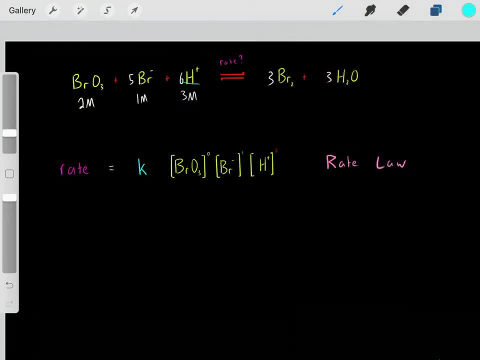 rate of a chemical reaction under certain conditions. For example, let's say we had these concentrations- two molar of this guy, one molar of this guy and three molar of this guy- What would be the rate of this chemical reaction? How could we determine the rate of? 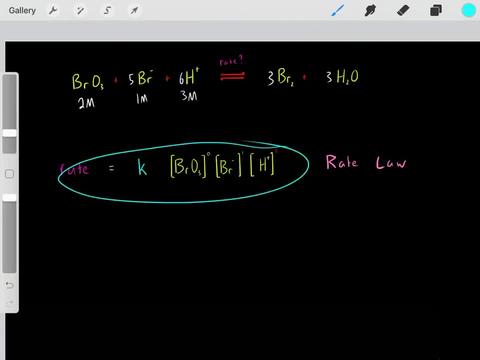 this chemical reaction? Well, we could just use this equation: We can determine the rate of the chemical reaction as long as we know the rate constant. And then we plug in the concentration of this guy here and it goes to the zero power. Then we put the concentration. 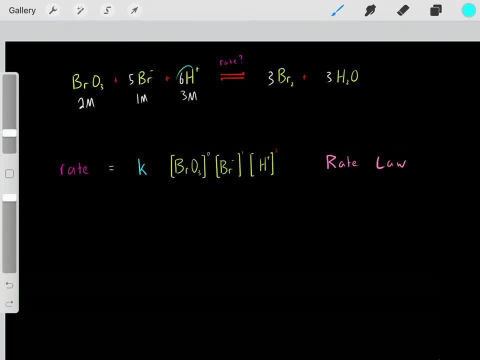 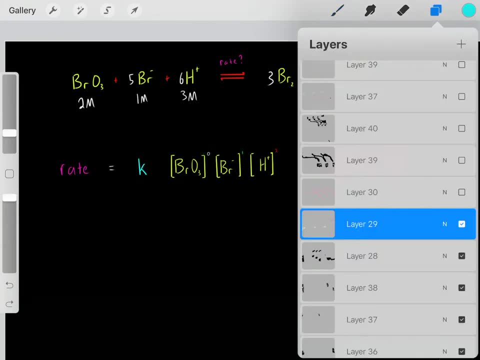 of this guy here and it goes to the first power. And we take the concentration of this guy, plug it in here and it'll go to the second power Because, again, this is zero order. This guy was first order and this was second order, So we plug in all our values. 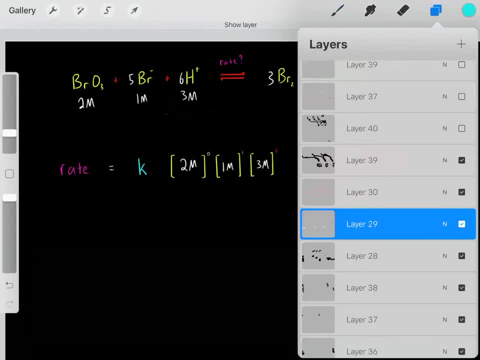 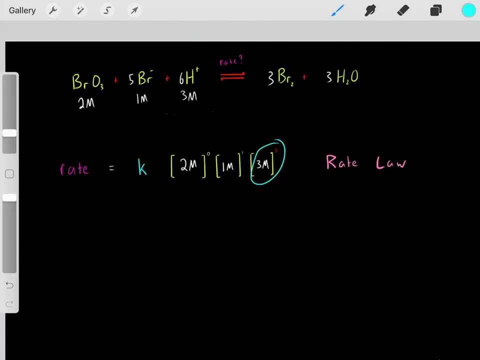 We plug in these concentrations. And if we plug in our concentrations it would look like this: Then we would just plug this in the calculator. Two is to the zero power. one to the one power. three, to the second power. Multiply this by the rate constant and that will tell you the rate of this chemical. 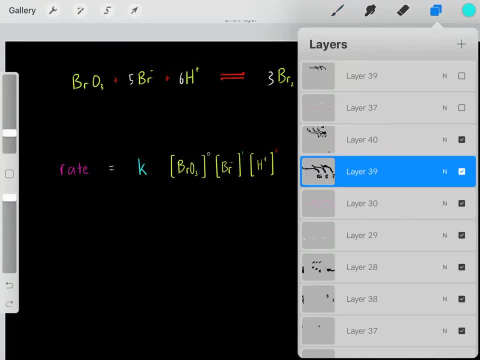 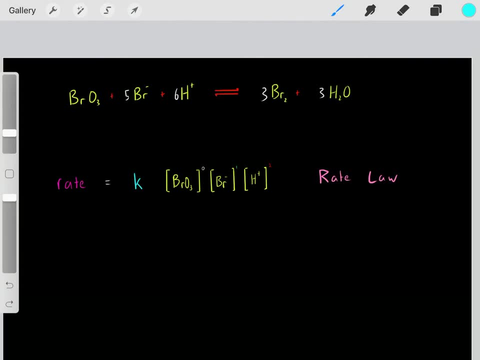 reaction using this rate law. So that's pretty interesting. But something important to realize is this rate law you can only determine empirically through doing experiments. For example, we know this guy's zero order. We can only determine that this reactant was zero order through doing experiments. When 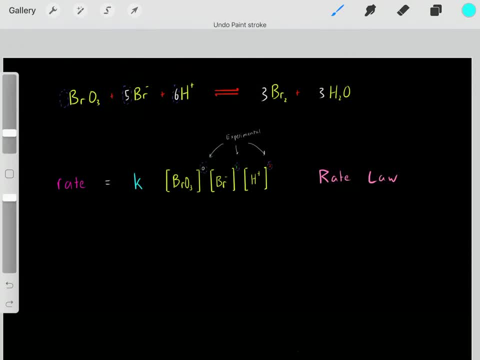 we do experiments and we double the concentration and we see it has no impact on the rate of the reaction. so therefore we can determine it's zero order. We know this guy's first order. through experiments, through empirical evidence, We double the concentration of this. 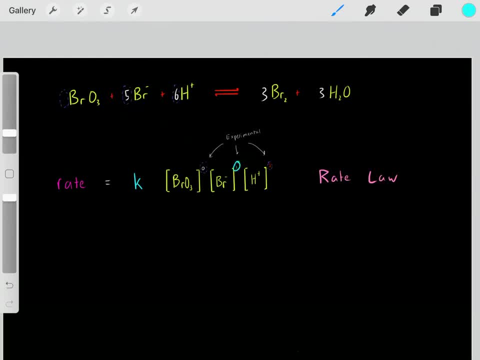 reactant, we double the rate of the reaction. so we know this guy is first order. Then again through experiments, we know this guy must be second order, so it goes to the second power. big mistake people make is they look at the coefficients of the balanced equation but that's. 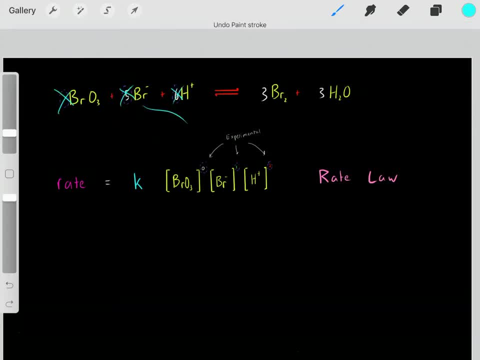 not important. that has no impact on on what order what, what order it is. so don't make that mistake. don't think that this guy must be fifth order and then you would put: you would go, this would go to the fifth power. no, that, these, these coefficients of the balanced equation, isn't what's important.